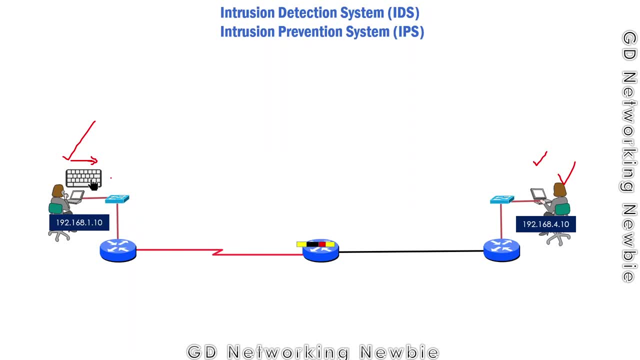 of frame is travels from one hop to another hop. now, when the data arrives at this route line and then the data is sent to the other hop, the data is then sent to the other hop. So let's take an example of this. for instance, in this case, at this router, we can see. so we are here and at this point in the network. 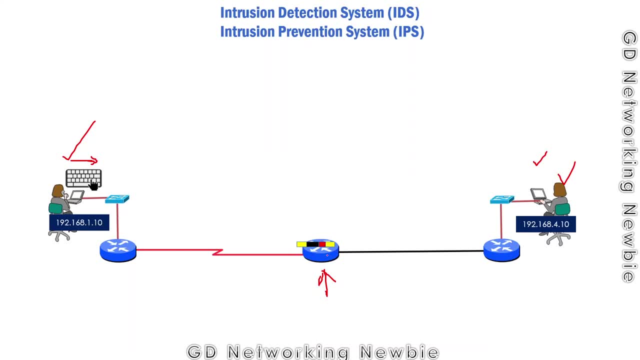 we want to monitor the traffic, so we want to monitor all the packets traveling through this router, because we we have some threads, some security threads, and we want to save our network, which is on the right hand side, so we want to monitor all the traffic flowing this routers. 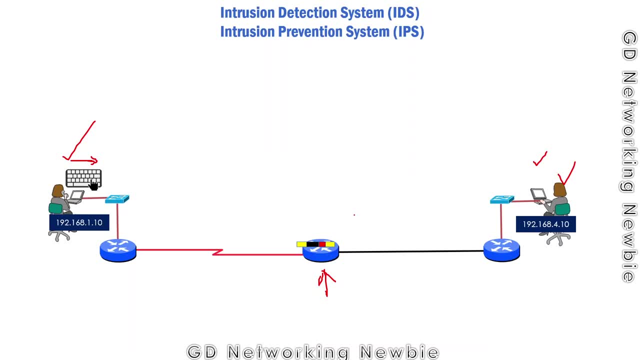 direction from this so we can close that. the router on the power. here we can provide some data. so this what we can do here: if we 우리가 maybe connect some of these minimal updates or lots or the latest updates or something similar to this, then we can continuously monitor those. this will be available in this table where we are. 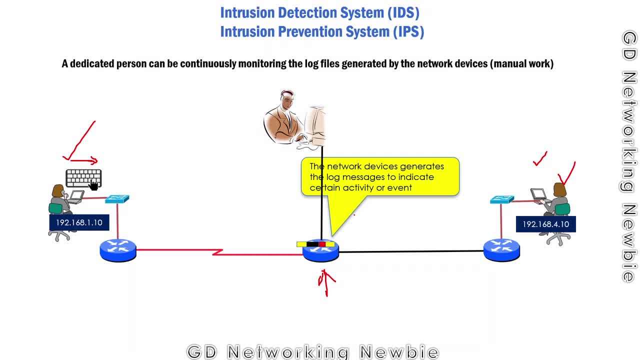 to send those log messages to some terminal where we will have a dedicated persons we can have like network administrator, who will be continuously monitoring these log files and in these log files, actually, this network administrator can find out some hints on the basis of these activity and events. 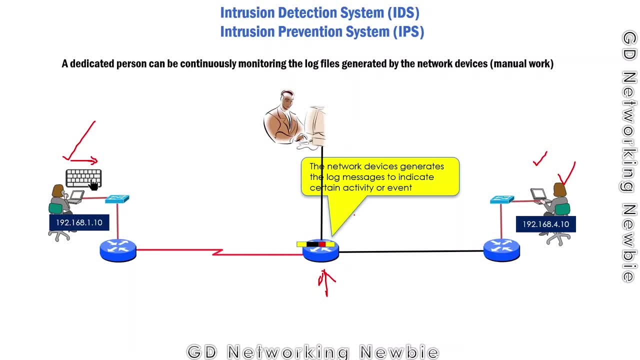 if there is any suspicious activity going on in the network, and on the basis of that log file this network administrator then can actually implement, may be the access control list or maybe some firewalls to save the network. no, so this is just display that these log files are generated on the 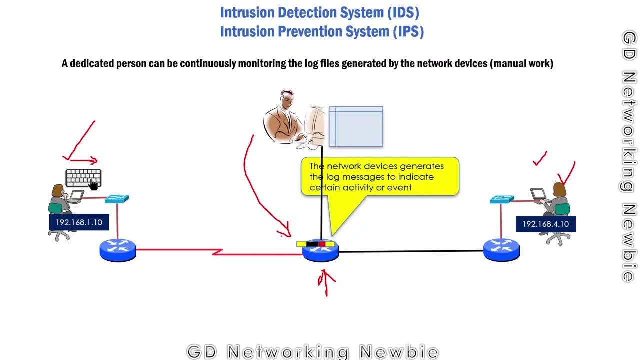 router and they are sent to the network administrator for further analysis of any potential thread. but this will be actually a manual work. so you see, this will be M méleod placed meeting status: manual work. It means we need a dedicated person to continuously monitor these potential threats. 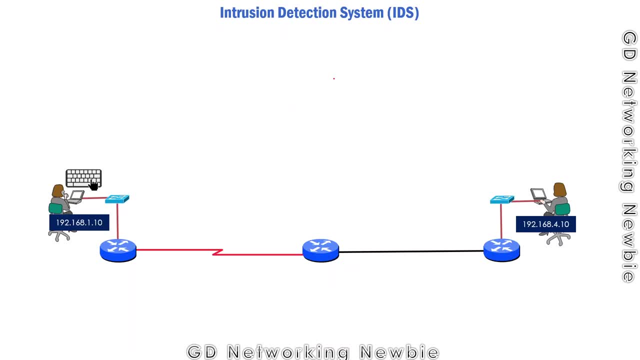 for the network. Now, let's suppose, if we change this scenario a little bit, So in that scenario, instead of a dedicated person, we are going to deploy or we are going to use a dedicated system for the analysis, And this system, dedicated system- is actually known as intrusion detection. 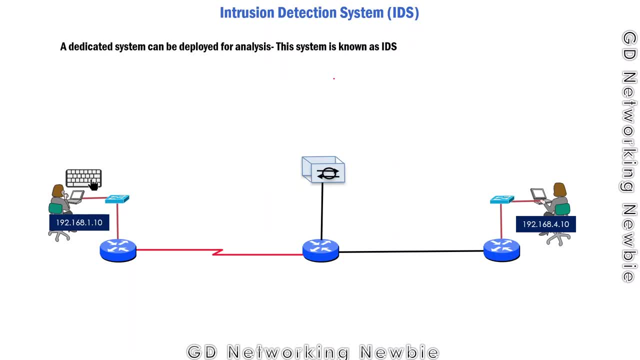 system So it will detect the intrusion. So in this case, what happens? if the user from the left hand side wants to send some data or some packets to the network on the right hand side? So when these packets arrive at this device, the device will be configured to send a copy of those packets. 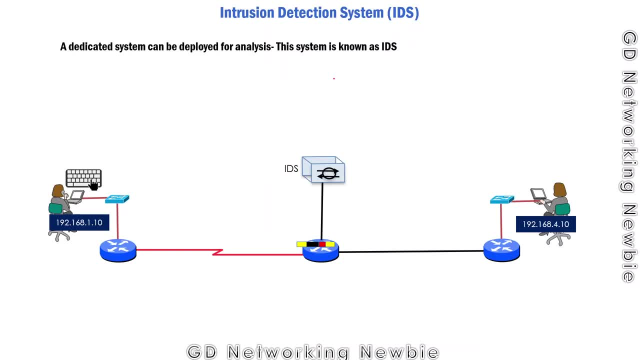 to this IDS device or this IDS system. So it means the one copy of the message will be sent to the destination and one copy of the same message will be sent to the IDS or intrusion detection system. And this intrusion detection system will also have a database of. 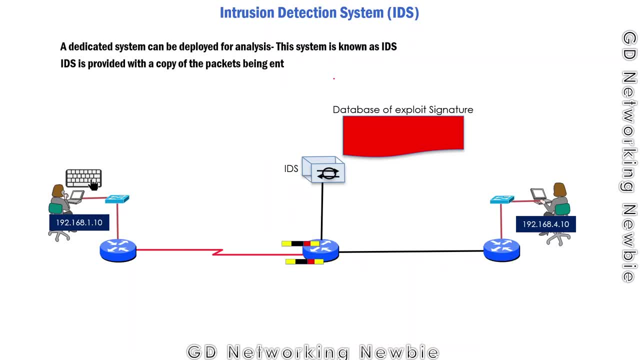 some exploit signatures. So signatures means some patterns, some hints about the potential threats. So for example, we can say: if you see the packets with some specific IP address or some specific packet with some specific keywords in it. So these kinds of information we can have in this. 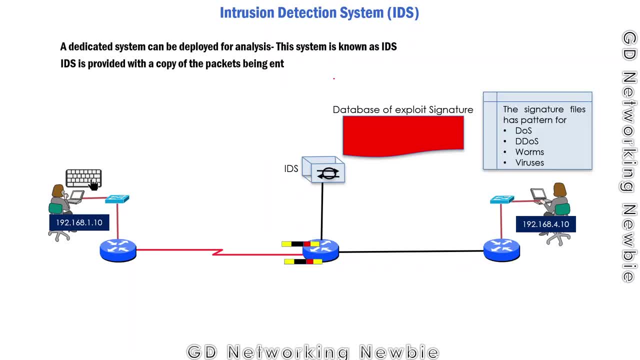 exploit signatures And specifically these signature files, actually has patterns for different kinds of attacks. So they will have hints to detect different kinds of attacks, like denial of service or distributed denial of services, DDoS or worms or viruses. So when the IDS 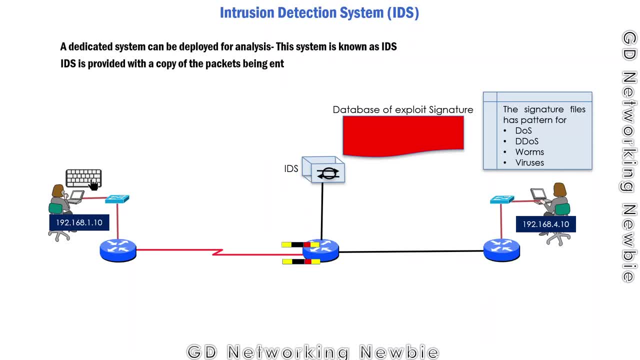 will have information about the attack, it will be able to detect the attack. So it will be able to have information about these signatures and this will have the packets as well. So it will run a matching process, So it will match those things, both of the things, And, in case of any, 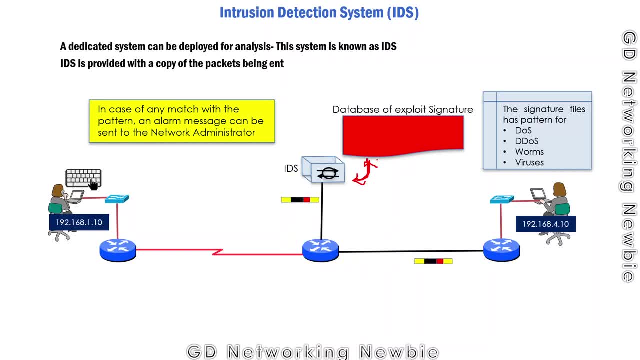 match with a pattern occurs, then this IDS can actually generate an alarm message and that alarm message can be sent to the network administrator. So in this case IDS actually is receiving a copy of the message and it's matching. So you can see the same pattern, but the pattern is not matching. 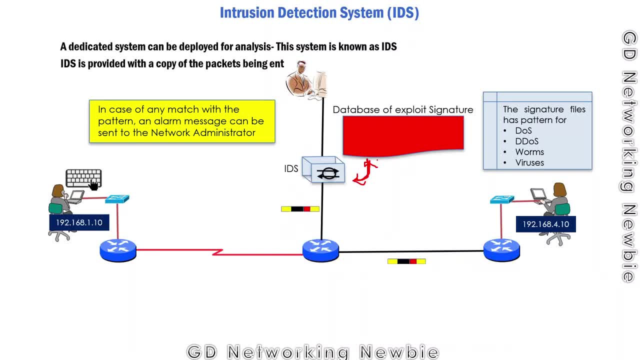 So you can see the same pattern, but the pattern is not matching. So IDS will also need to send some initial notifications and that's a huge advantage of IDS. So if you just take a new signal and if you matching that message with the, with the potential threads or the signature of the threads, or the 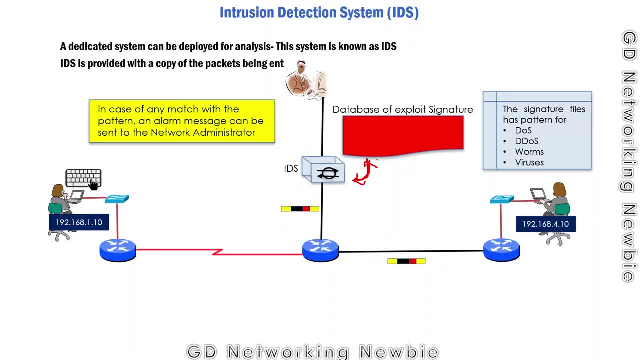 patterns of the threads and, if it, if there is any match, this information or this alarm message will be sent to the network administrator. but the important point is that that ids will not take any action. so if, if there is some problem, if there is any match, it will just send the alarm message. 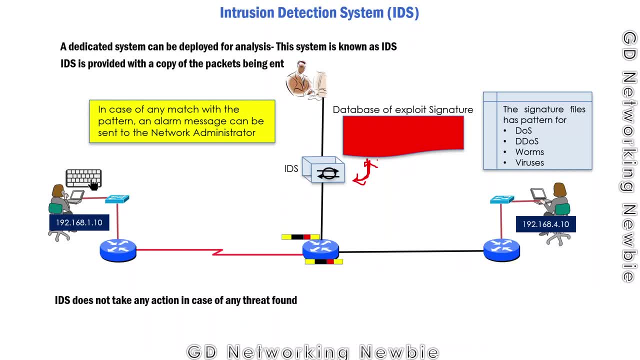 to the network administrator, but it will not take any action. it means it will not block the traffic or it will not discard the traffic. so this, this, the, the- i mean this will not be the- uh, a job of this ids to take any action. so this is all about ids and let's move to ips. so that's inclusion. 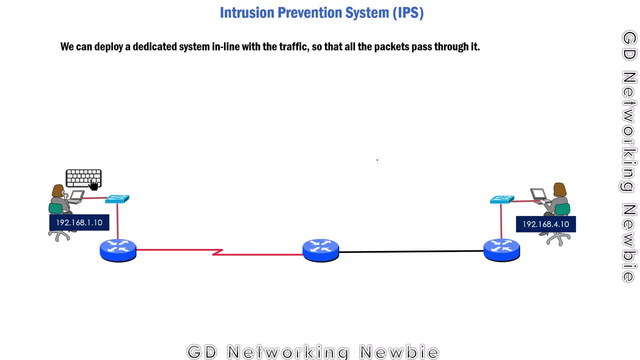 prevention system. so in this inclusion prevention system, we deploy a dedicated system, but this time that dedicated system will be in line with the traffic. you see, here we have deployed an ips, a dedicated system, and that's in that, and in line means that all the traffic which is coming from 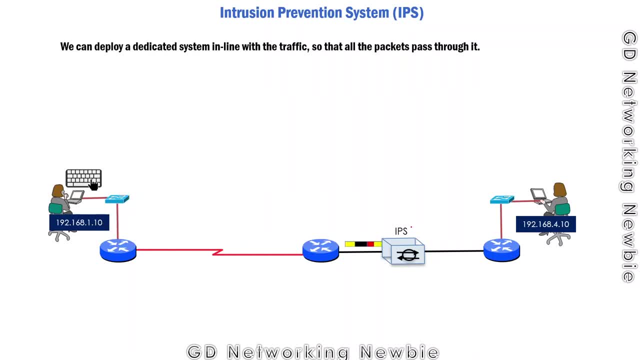 the left hand side network will be flowing through this ips. so it means every packet which has to be sent to the, to the network on the right hand side, that packet has to flow through this system. and this- i this system will have a database of exploit signatures- means this will have a pattern. 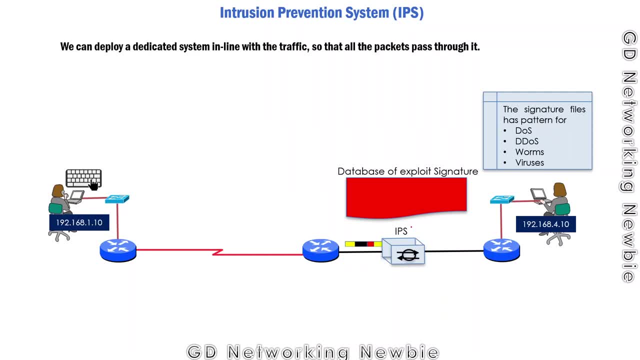 of potential threads. in the same case we can have the pattern for different kind of attacks there. so every packet which is flowing through this system will be matched with the pattern or with the signature of potential threads and in case of any match with a pattern, a predefined action, 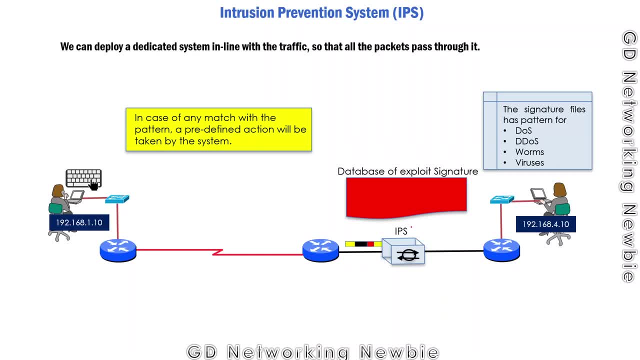 will be taken by the system. so the difference is that in this case, system is going to match the packets which are traveling through this system with the signature or the pattern and if there is any match, and if there is a match for any potential thread, then this ips can be configured to take certain action. so action means maybe it will not allow. 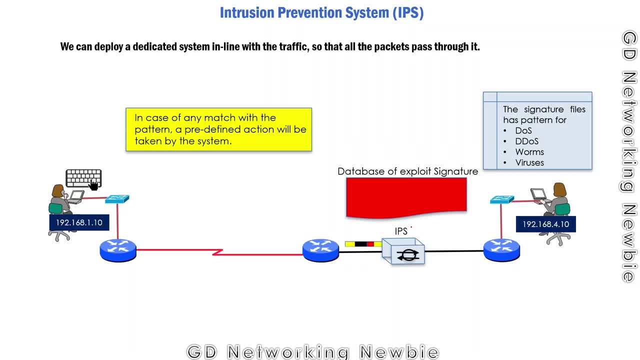 that particular traffic or that particular packet to go through that system. it will just discard it. maybe it will block it. it means, in addition to detection, it's also going to perform some action. so it means it's going to prevent our system from some potential threats. so this is the 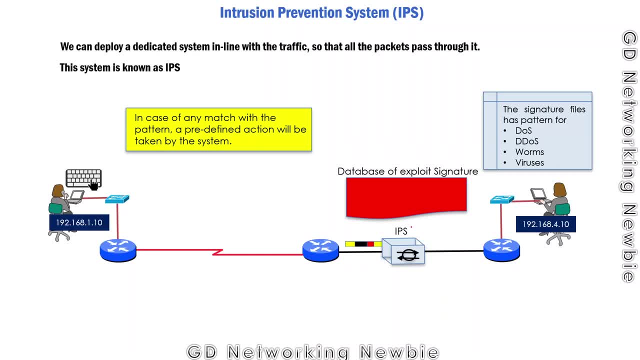 main difference between ids and ips. now this system is actually known as ips intrusion prevention system, because it is not only detecting, but it's also preventing our network from some potential threats. and then the question comes that from where we get these uh database of exploit signatures, where we have the patterns? 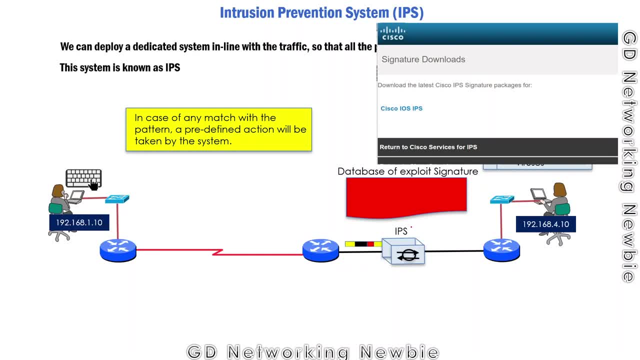 of some potential threads where we have the hints about some potential threads like denial of service or some viruses or hide. so who is going to give us these signatures, the database of signatures? so this database actually comes from the vendor, so the vendors of ips, for example. in this case, if 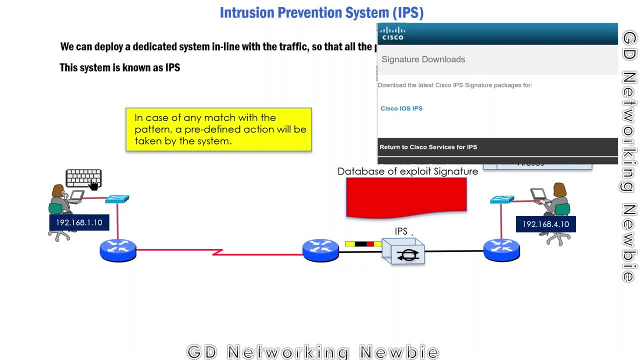 we have IPS from Cisco, then Cisco will provide us these files and we can go to their website, like ciscocom, and we can have the signature downloads section there. we can download these signatures and we can, we can have download these signatures in that specific device. and then this: 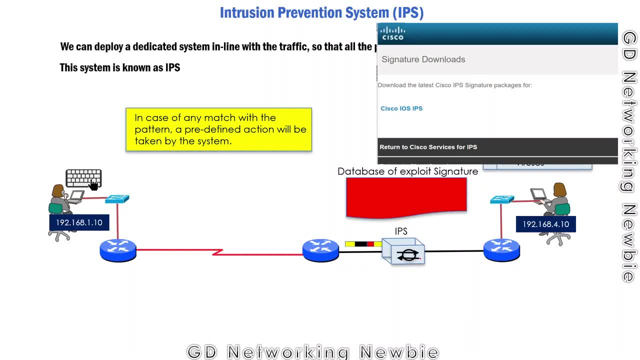 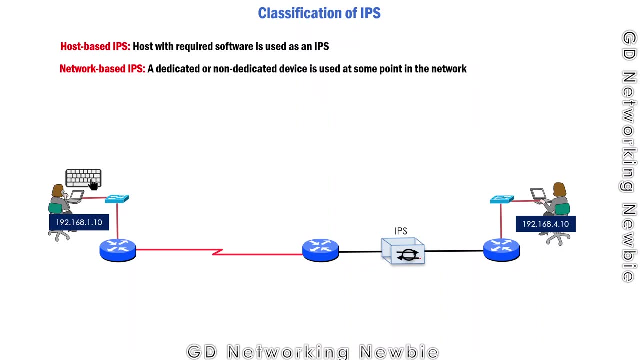 device can be deployed in line with the, with the packets, and we can. we can get the performance or the actual job of IPS and we can secure our network in this way. so this is. this is some information about IPS. now these IPS can further be classified or we can say there are different. 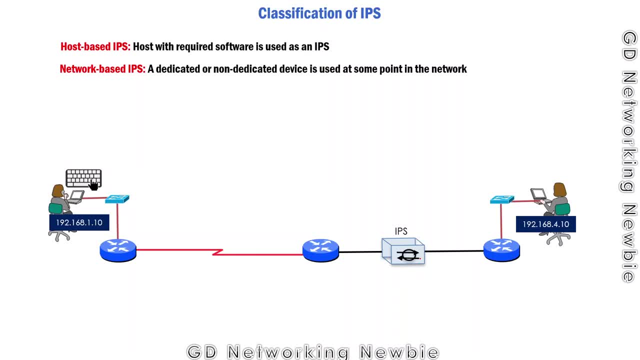 kinds of IPS. so this depends whether we we are going to deploy that IPS functionality on host, so that is known as host based IPS. and in this host with IPS, actually host will be, will will have a software and that software will be acting as an IPS. so in this case, for example, we 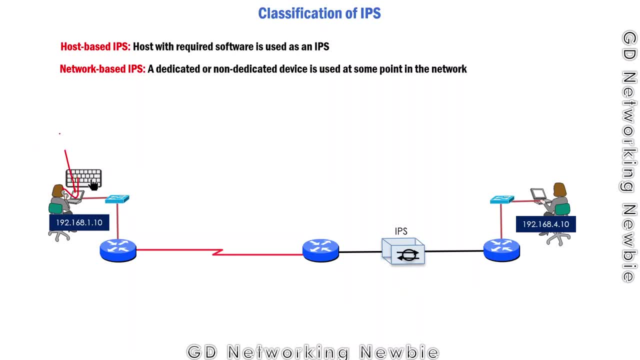 have this computer. this computer can have IPS software there and it can check locally about the threads and we can also have network based IPS. so network based IPS like we have this one. so now this is there to save not only a single host, but it is there to save the network as a whole.